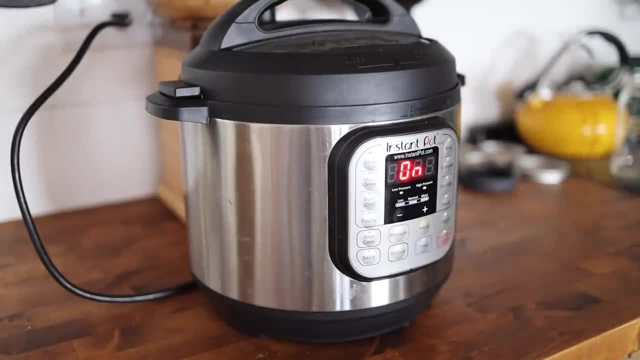 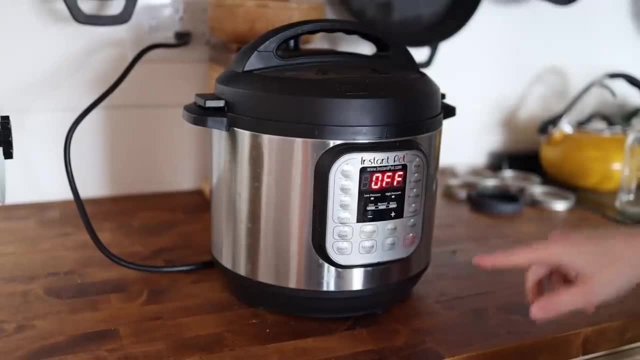 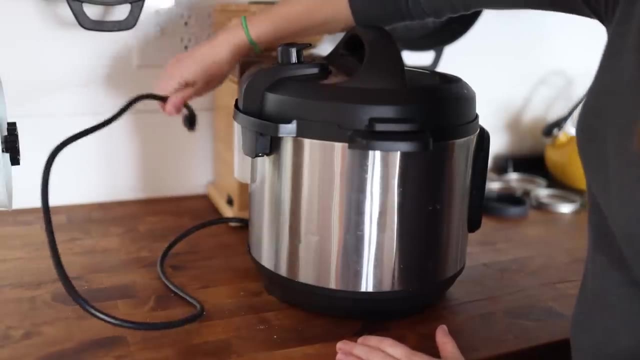 probably our number one snack food that we always have on hand If it is between meals and someone's hungry. they know that they can always go and grab a hard-boiled egg. and I love that. it's high in protein, it's nourishing, it's satiating, it keeps you full. 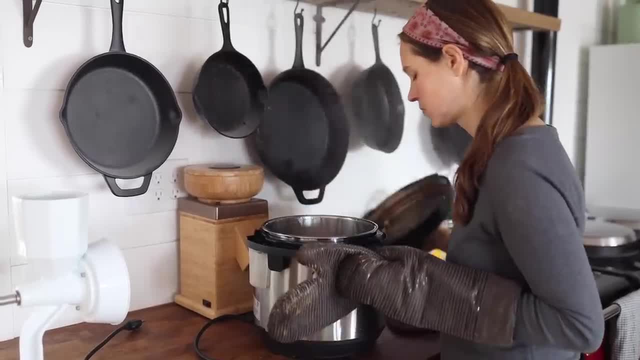 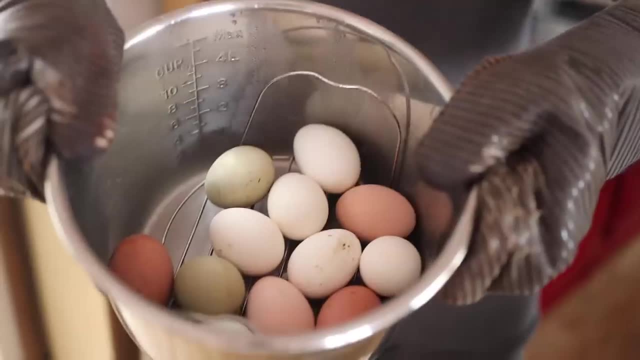 and longer, and it nourishes little bellies and big bellies. So that is just one of our staple things that we always have on hand. It's also great because our kids can quickly make them for breakfast for themselves. They don't rely on me to need to make them for breakfast. They don't. 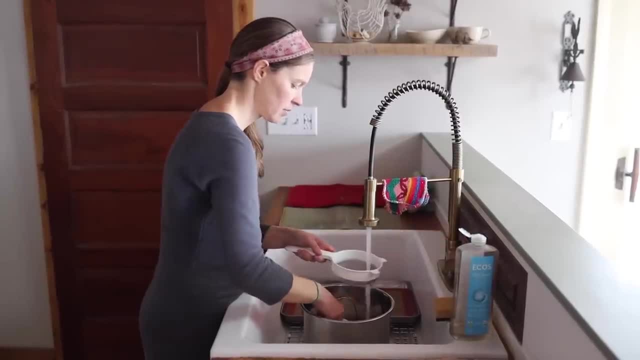 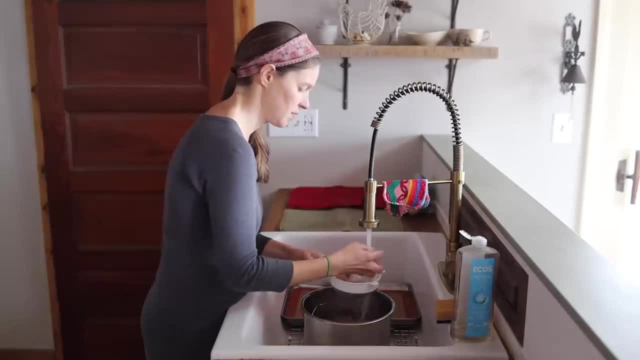 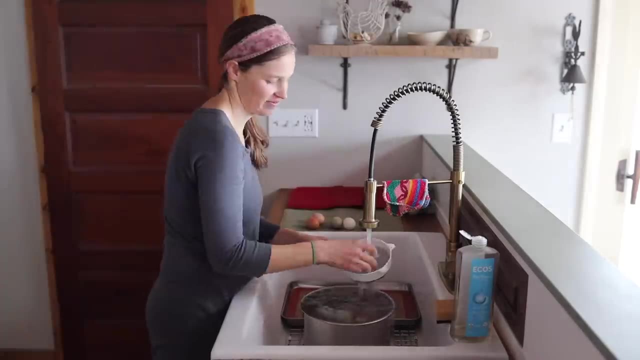 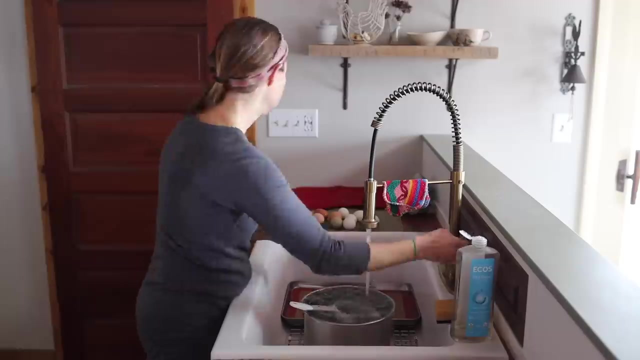 I'm not available. hard-boiled eggs are great. I love to make them in the instant pot. You can also make them on the stove, but I have found that the instant pot is just the best way to make them, so that those shells just slip off super easily. I've never found another method that works as well. as the instant pot, and so I do it at a manual high pressure in the instant pot for five minutes And then I let them naturally release for four minutes after that and then I quick release it, pull them out, and you want to get them chilled as quickly as you can. So you can do this by putting 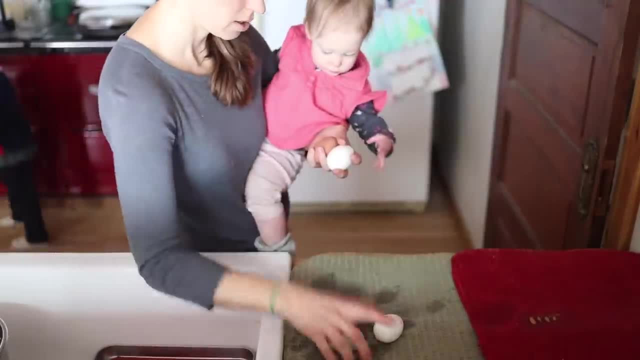 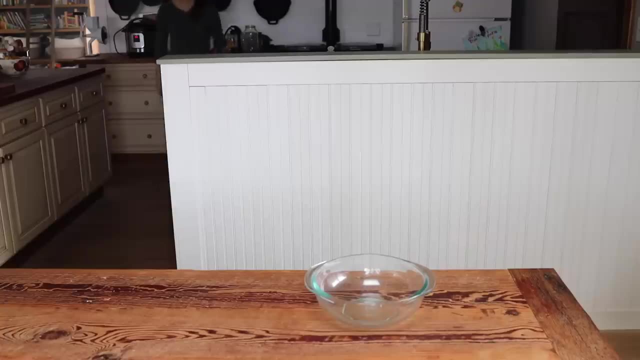 those hard-boiled eggs in an ice bath and chilling them down that way- or I just generally put them in a strainer and put them under as cold of water as our frost it will go- get them chilled, dry them off and then get them in the fridge as quickly as possible. 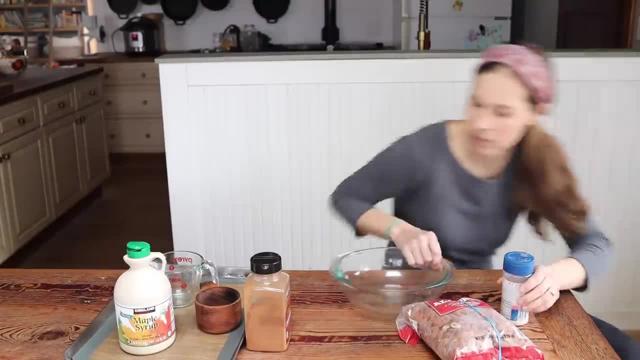 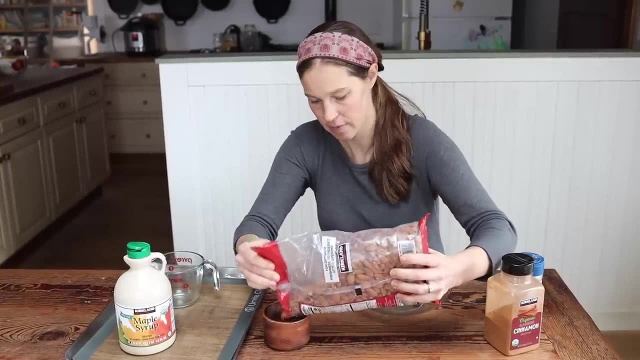 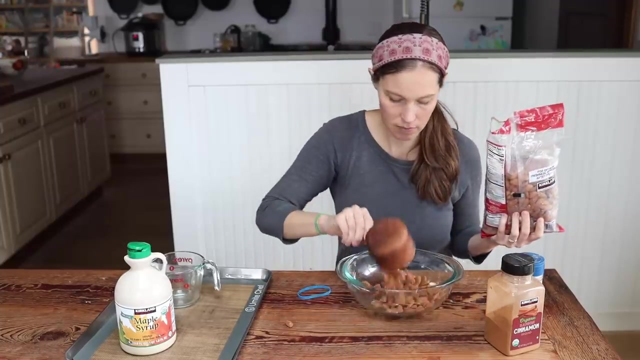 We recently had a birthday party for our daughter with her friends, and she requested a charcuterie board for their party, and so we wanted to have nuts at her charcuterie board, and so we made these maple spiced almonds, and they were such a big hit. Everyone loved them, and so they have. 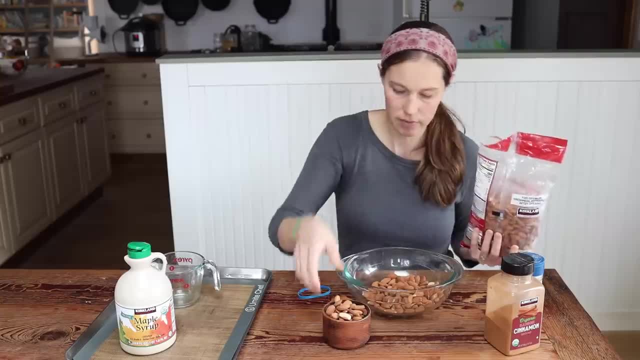 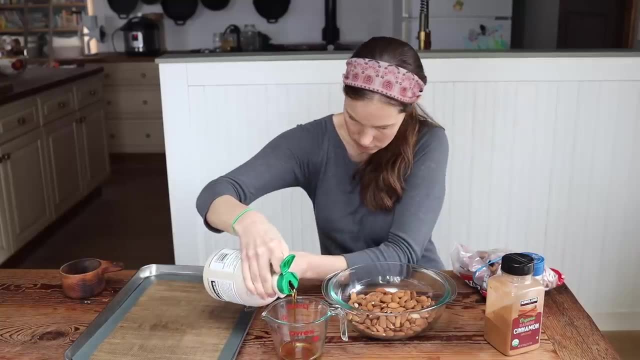 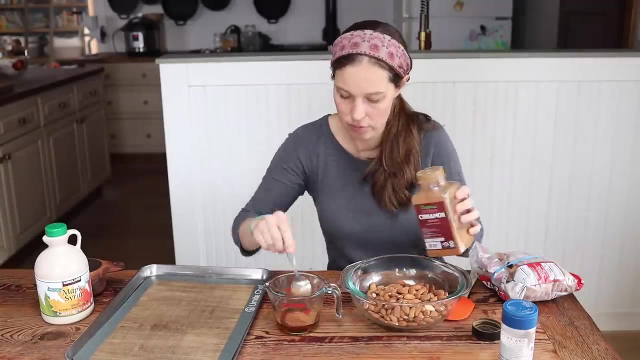 since become a staple for us. I had already liked to have nuts, maybe some raisins on hand. they're just a really great, easy grab and go sort of snack food that gives you good nutrients: There's protein, there's fat. they're also like the eggs gonna keep you satiated and 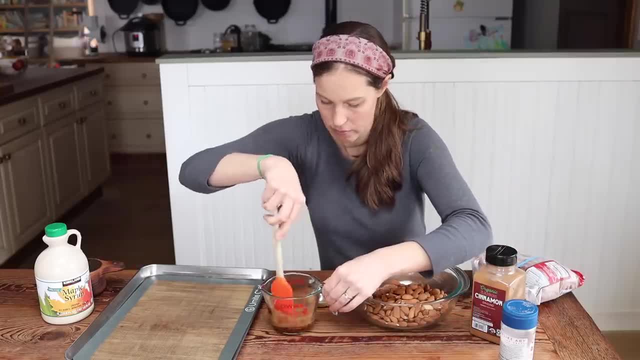 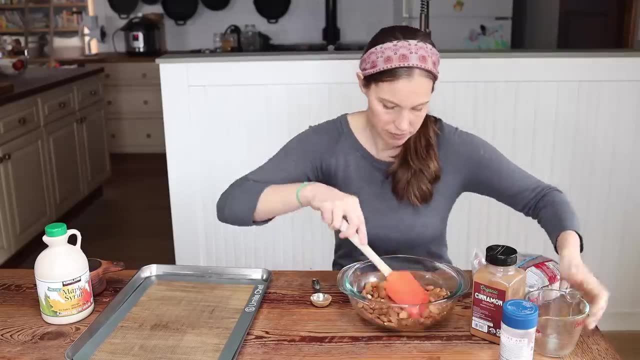 just has better nutrients than a lot of packaged snack food. but adding the maple syrup and the cinnamon just really takes them up to the next level And they're really really easy to make this way. I'll post the full recipe below, but the basic idea is that you just take. 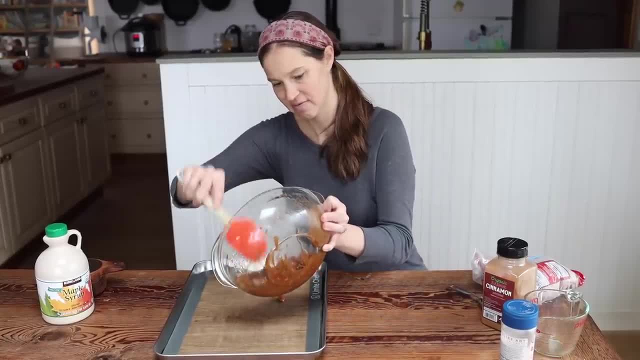 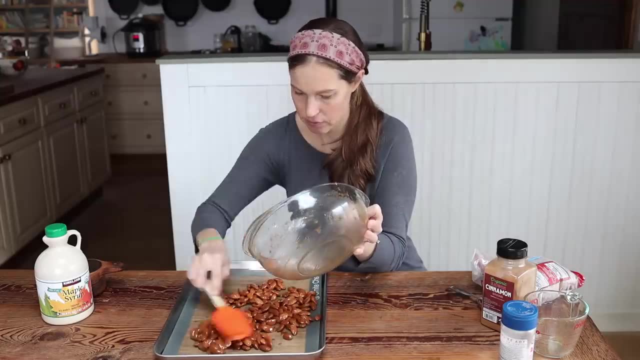 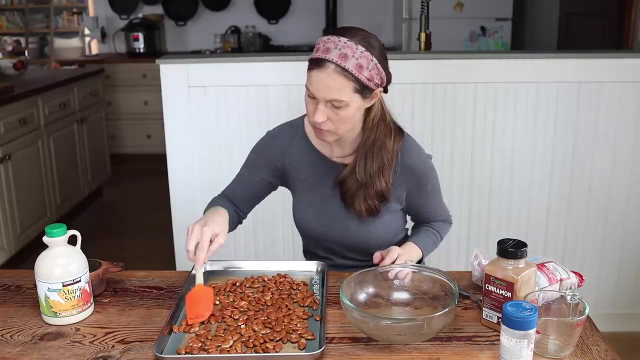 a bag of��. i'm using almonds in this recipe, so take a couple cups of almonds, add a little bit of maple syrup, some cinnamon and some salt, mix that all together, lay it out in a single layer on a baking sheet and then bake them at 350 degrees for 15 to 20 minutes. 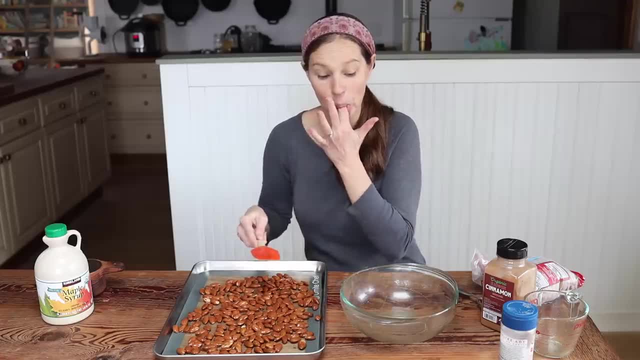 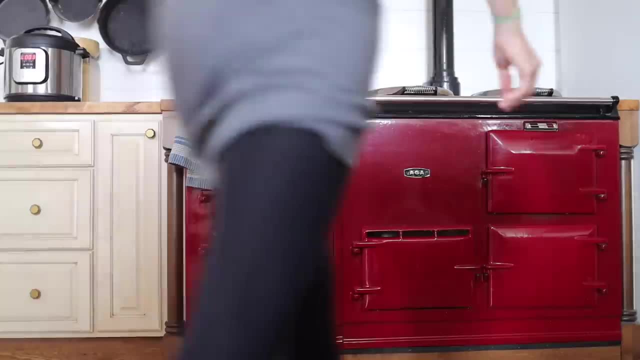 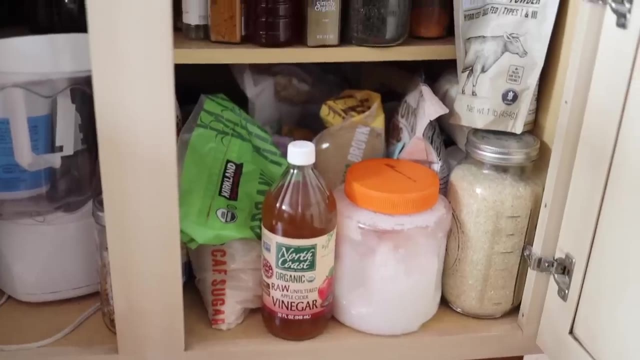 let them roast up and break them apart and they're ready to go. these almonds are also really great, because not only are they good for on the go, but they would also be really yummy on a salad or something like that. so here's a little snapshot of our very 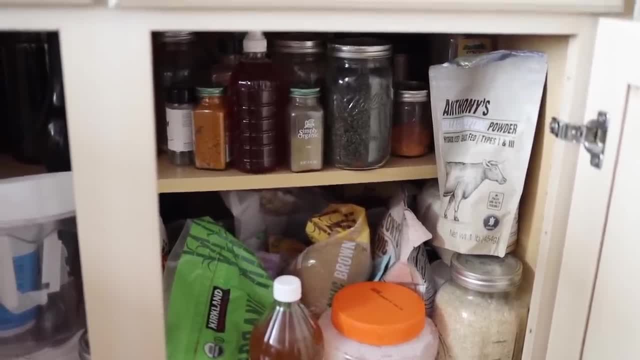 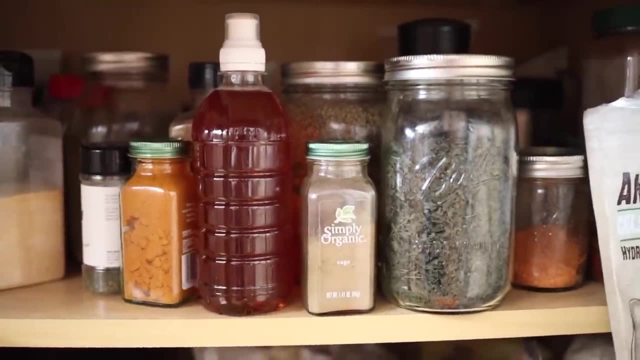 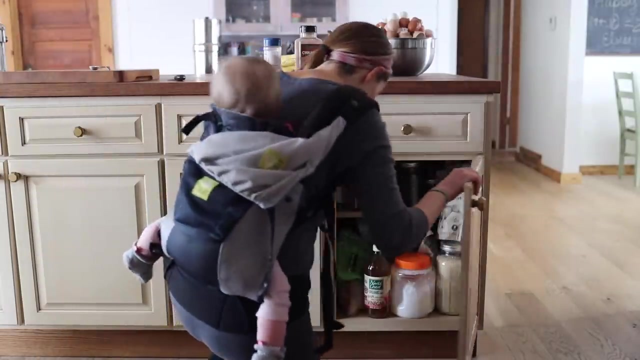 not clean real life pantry and, as you can see, there's not a lot of packaged snack foods in our pantry. it's basically just a small lower cabinet in our kitchen where we keep all of our dried goods: spices, oils, vinegars, some different flours and baking. 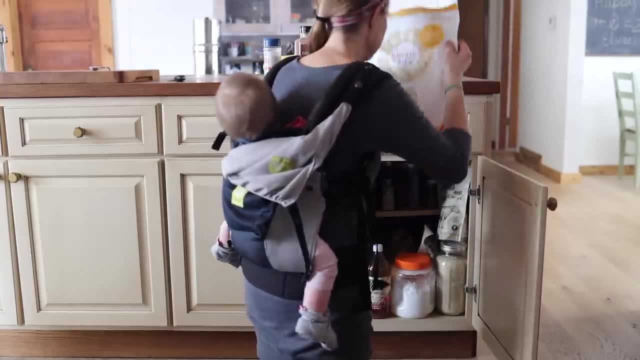 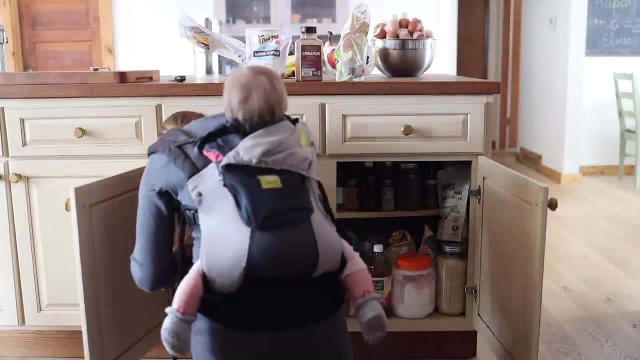 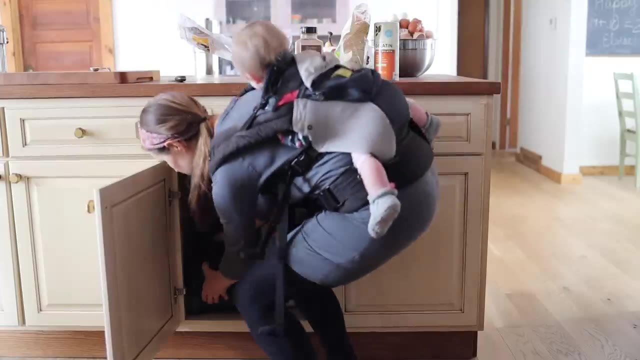 things, things like that, And I am not opposed to like ever buying packaged snack food from the store. However, we do rarely do it, but on occasion, if we're traveling, it might be helpful to pick up a couple Lara bars or something like that. However, I have found that when it comes to 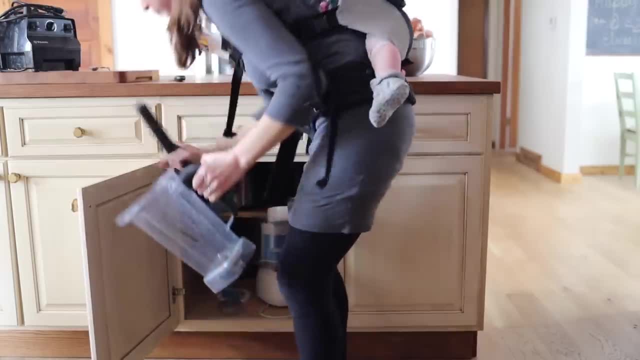 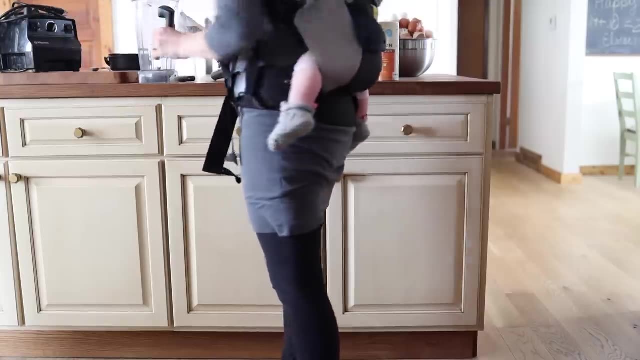 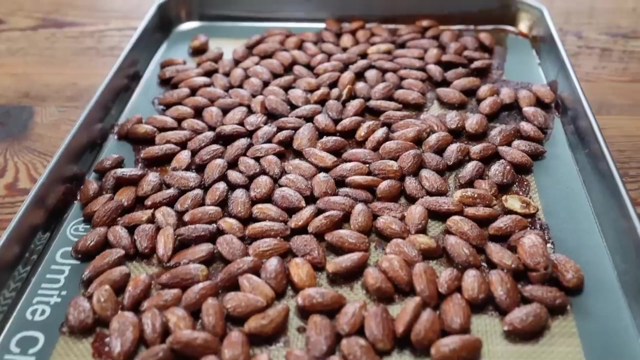 packaged snack food. it's really hard to find things with good quality ingredients, especially without having refined oils in them. It's just really hard to know what you're getting. There's just not a lot of transparency when it comes to packaged food. And then the other thing about it. 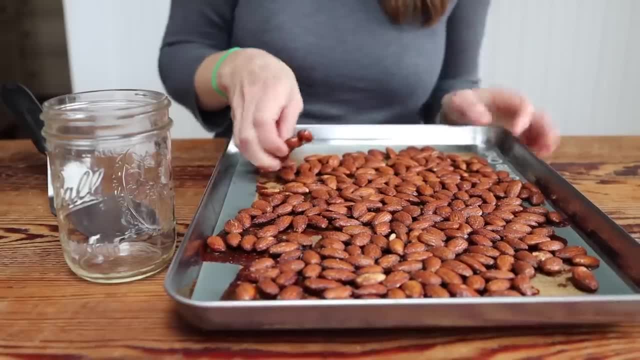 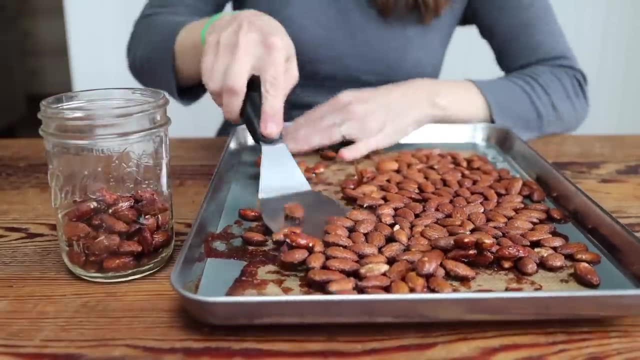 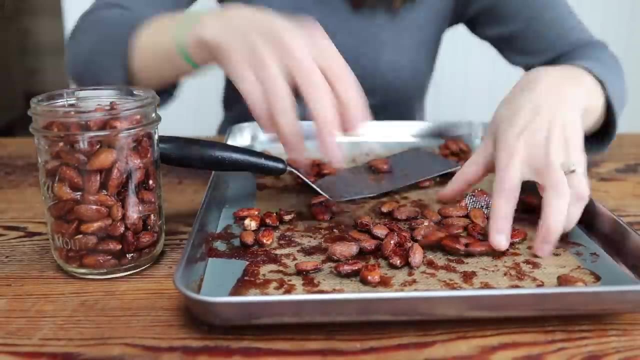 is they're really, really expensive. So, while it can be very convenient to buy packaged snack food, it's not going to be very nutritious and it's not going to be friendly on the budget, And so we have found that it's really pretty easy to make a lot of these things at home, and it doesn't. 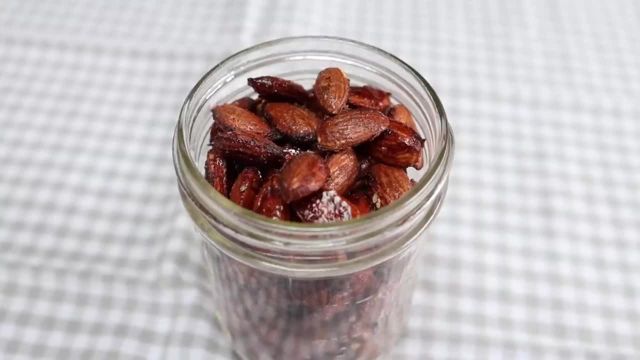 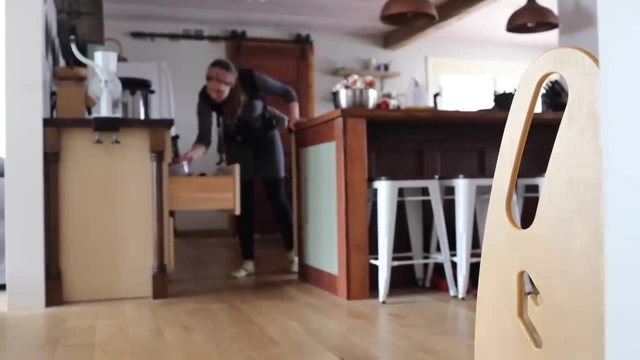 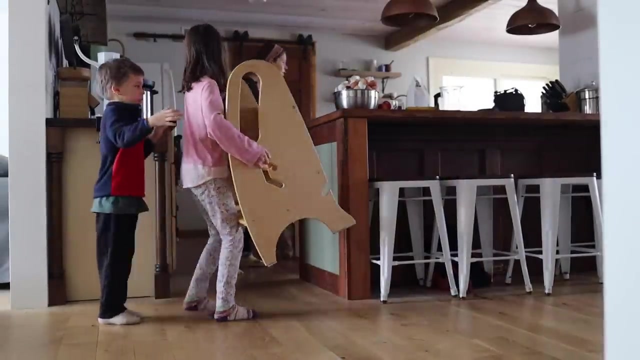 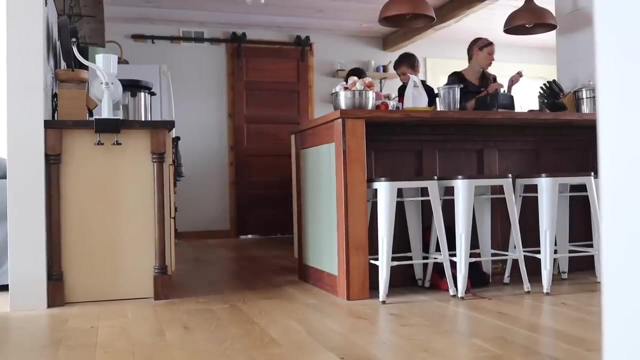 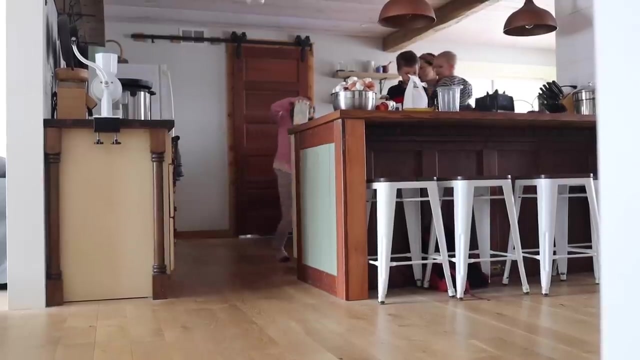 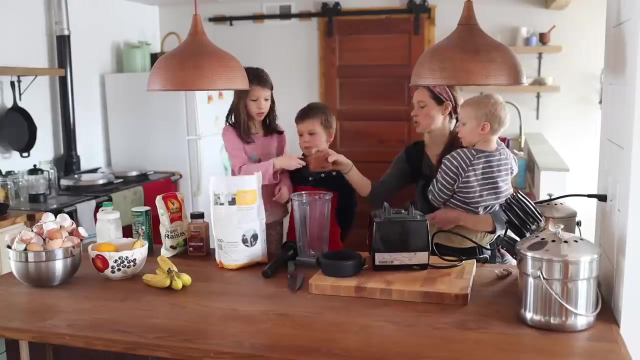 have to take a ton of time and it saves you a lot of money. With the nature of our world being a kind of primarily home-based family, we honestly just don't do snacks very often. So our world is home, We homeschool and we. 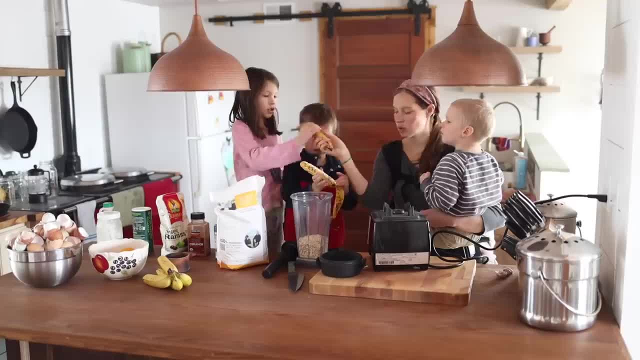 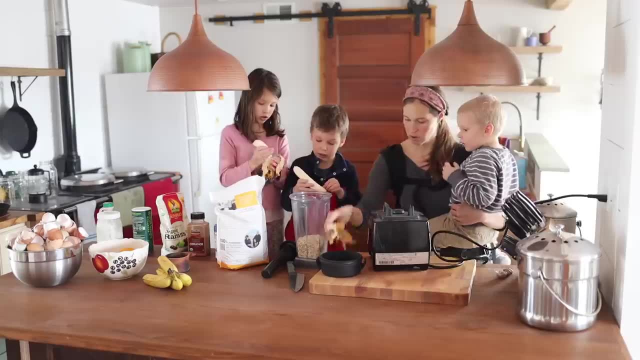 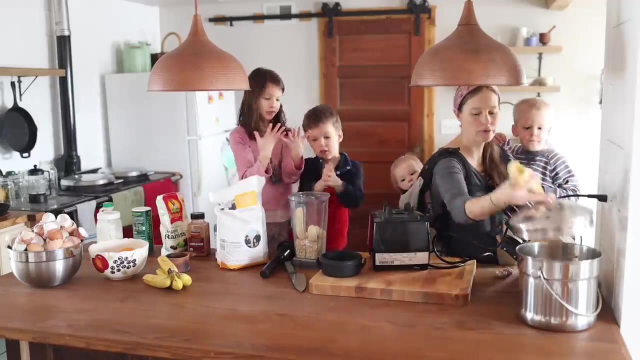 homestead and we are just here most of the time, And so most days look like we eat a solid breakfast and then four or five hours later we eat a solid lunch, And then four or five hours later we eat a solid dinner, And most days there is really no snacking. that happens, However. 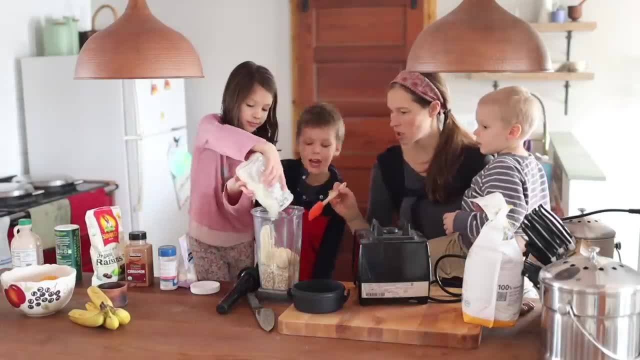 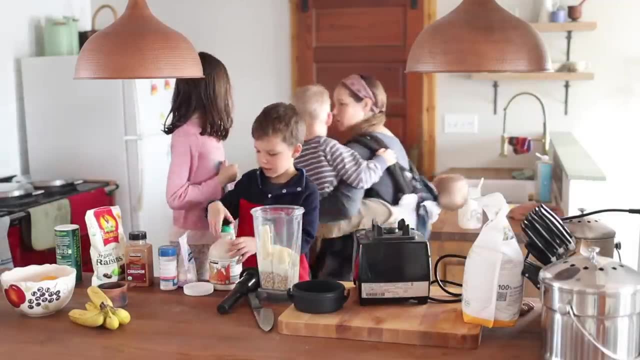 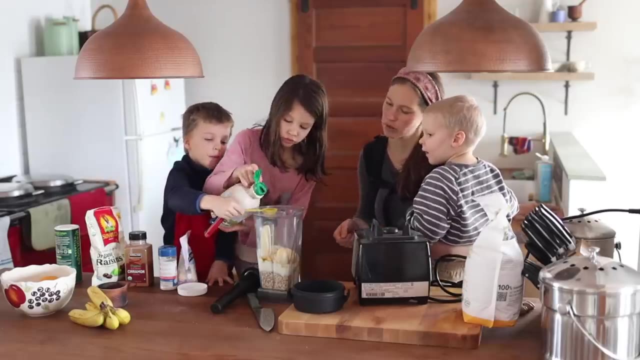 I like to have a few of these things on hand, because you just never know what might come up, And occasionally we have days that aren't at home. We have days that we're at our homeschool co-op, or we are going to run errands for a half day, or we're going to go on a hike with friends and 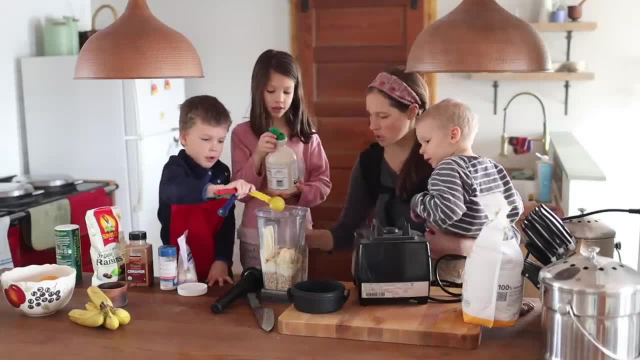 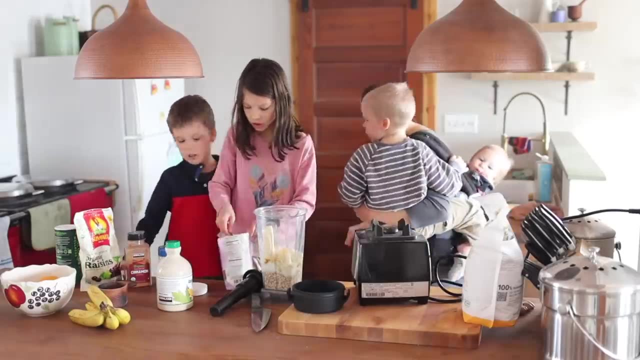 it's good to bring something with you. So for us, these things like we're making today are more of a good to have on hand for those situations when we do have to run out and are gone for a good chunk of the day. But on occasion too, there are days when we are. 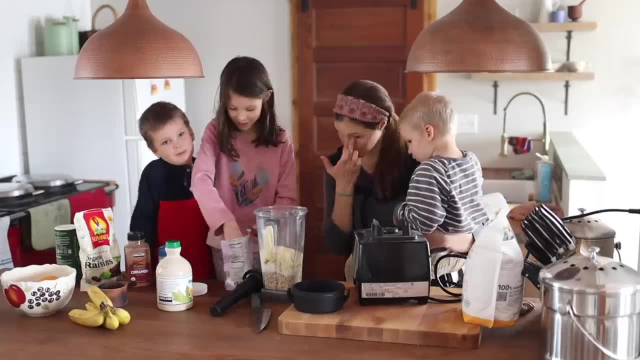 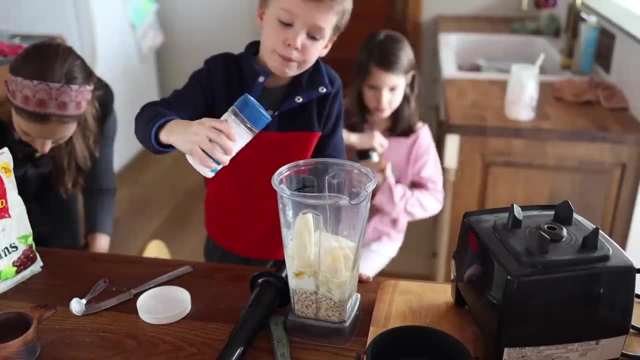 here, and it's just, someone needs a little. pick me up in the morning or in the afternoon, And then it's also really nice to have these things on hand. Sprinkle a little salt, sprinkle a little cinnamon, and then we'll blend her up. What do you want to put in buddy? 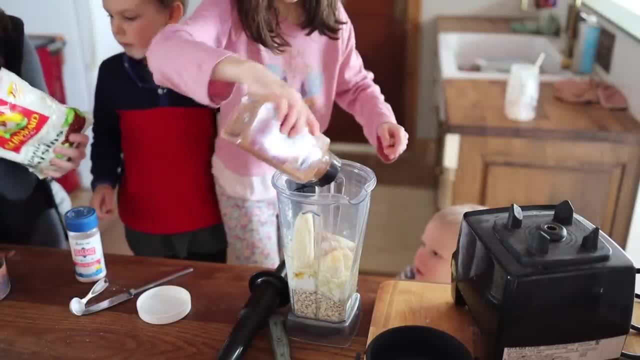 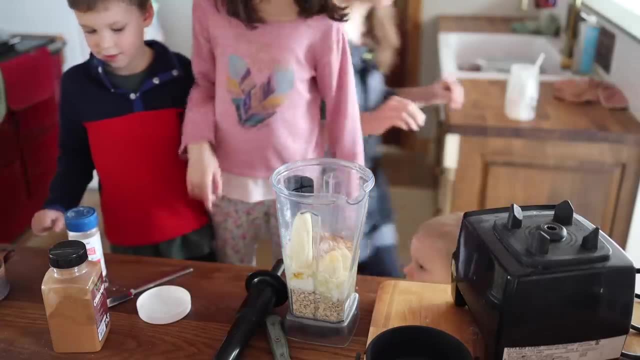 The raisins come after. We have to blend before we put the raisins in. Oh yeah, we don't want to blend the raisins. We don't want to blend the raisins. Is that good? Now we're going to blend. 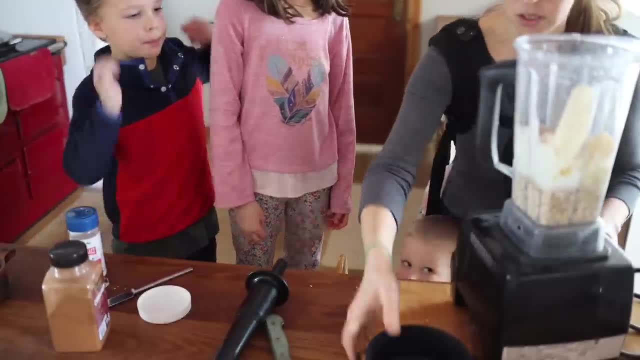 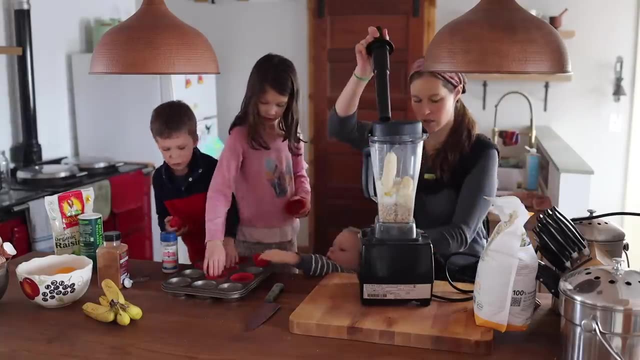 Our kids have been asking to make these banana oatmeal muffins for several weeks now. We've made a few different kinds of muffins over the years, but these banana oat ones are just the go-to ones that they keep requesting over and over again, and a favorite in our house. 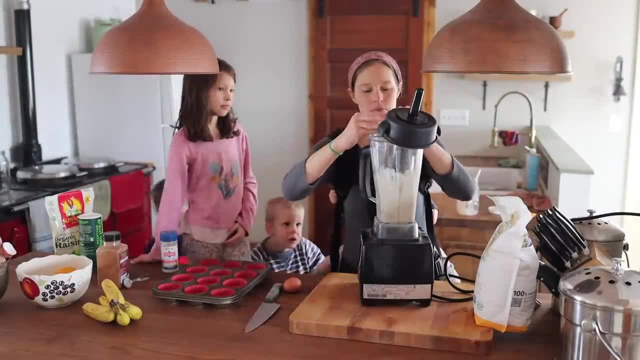 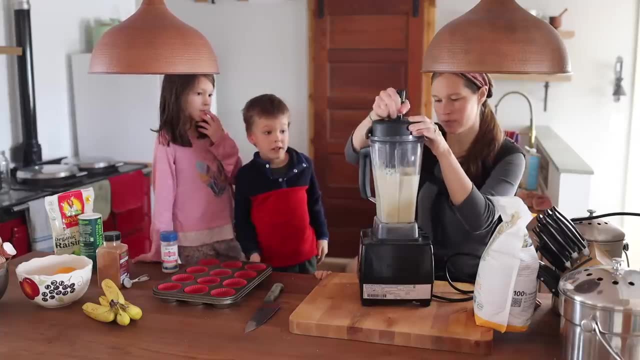 And so we just happened to have a couple extra bananas on hand that need to get used up, And so we are going to make these banana oat muffins today. The recipe is below, but I like them because they really only involve a few six or seven main ingredients. 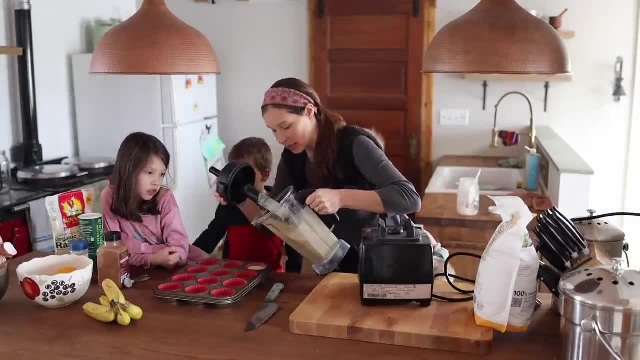 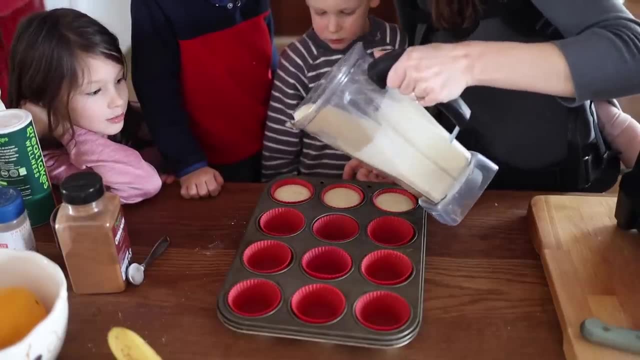 like oats yogurt, your bananas- no extra flowers, just a little bit of maple syrup as a sweetener along with your bananas. So always things that we have on hand and they're so easy to make. Our kids can just put all the ingredients into. 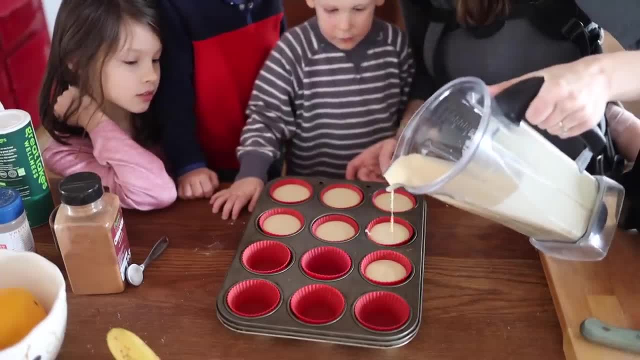 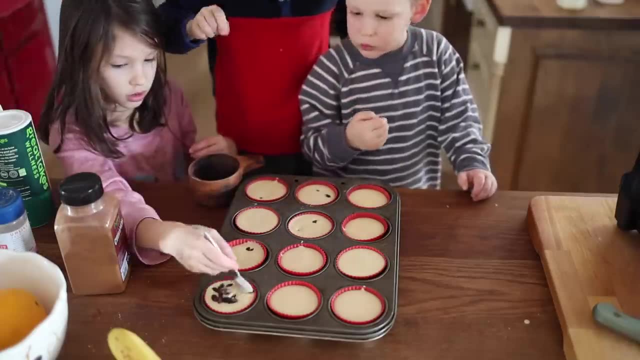 a blender and then you're going to turn the blender on That makes the batter Pour those into muffin cups and then you can add whatever mix-ins that you want. You could add chocolate chips, or our favorite way to make them is to just add raisins to make a banana raisin. 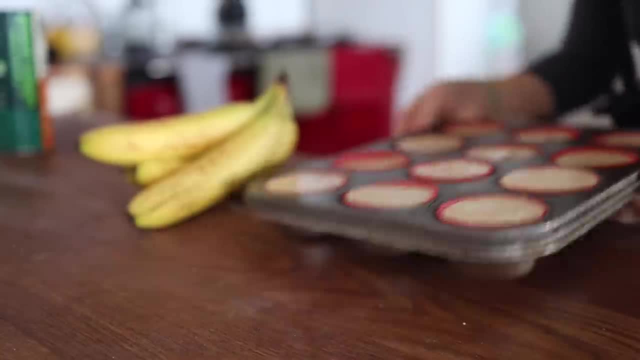 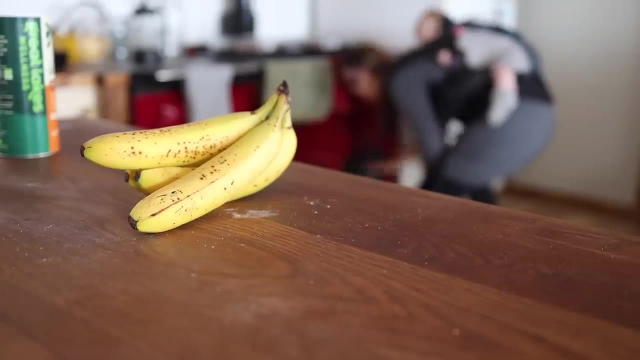 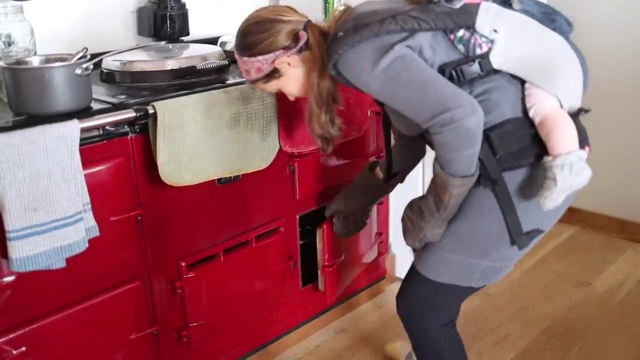 muffin. So when these muffins come out, I'm just going to store them right away in the freezer, And so to do that, I take them out of the pan and I flash freeze them on air, And then I put them in a lined cookie sheet and let them freeze in the freezer And then 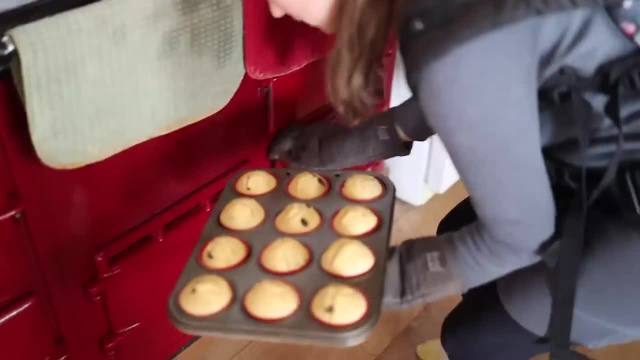 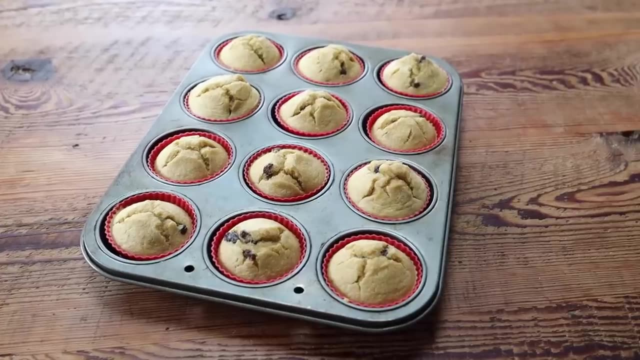 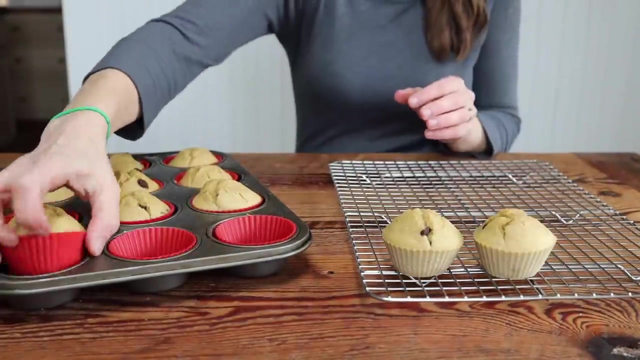 once they're all frozen, I take them out, I put them in Ziploc bags and store them in the freezer, And I like to do this because then I can just pull them out whenever I need to. It's so nice to just have some muffins ready to go in the freezer, So if we are going on, 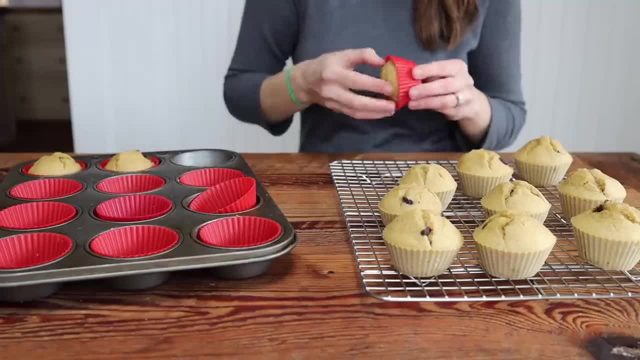 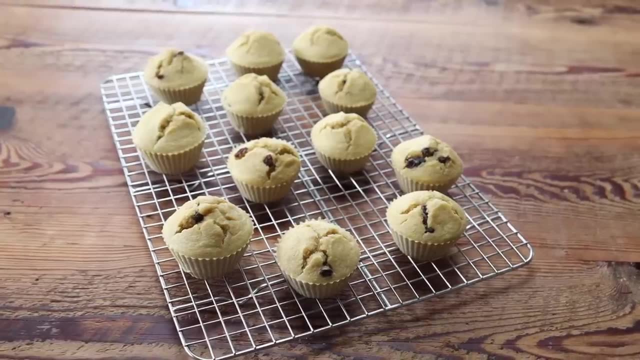 a hike with friends or I need to pack a lunch to take to co-op, I can just grab a couple muffins, one for everyone, And it's really cool. They're really, really delicious. So and add it to what we're bringing, it'll thaw in the way. 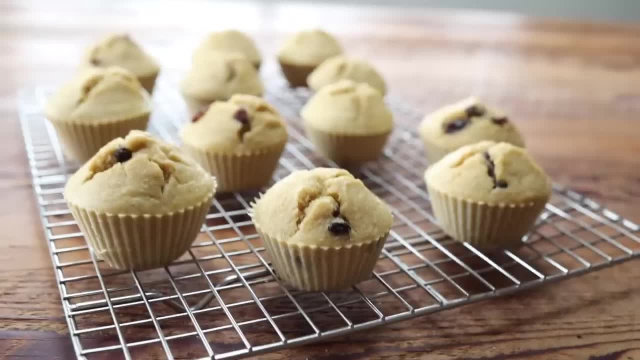 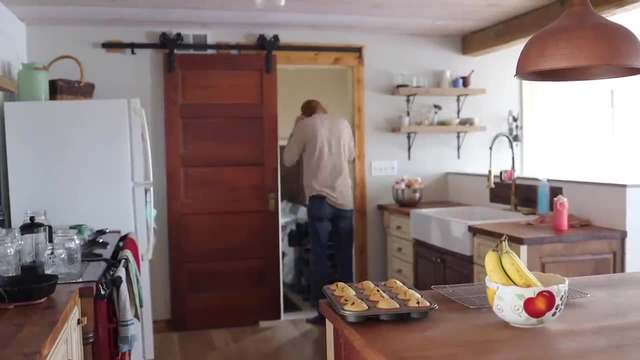 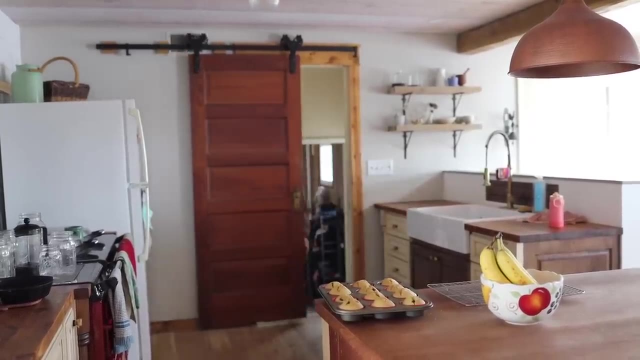 and it's just super easy: done, ready to go. You may have noticed this really large bowl of eggshells sitting on our counter that is overflowing, and so Jim is gonna go run this out to the animals. We always have a bowl of eggshells collecting on our counter. 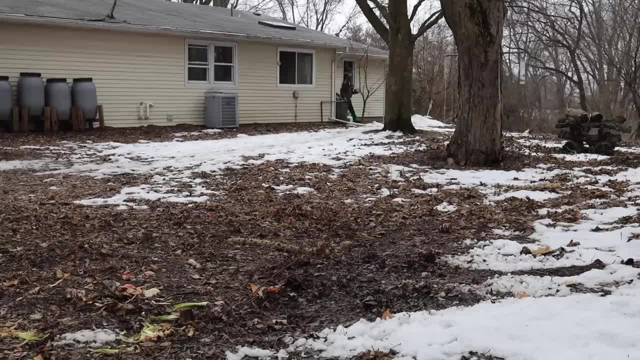 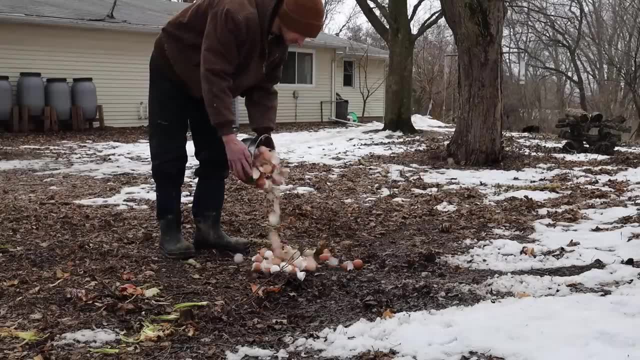 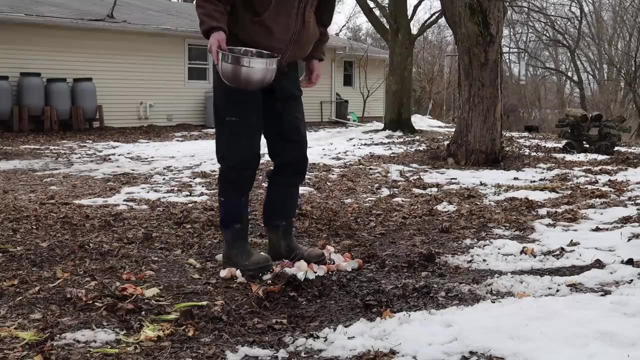 that we go ahead and give them to our chickens, or sometimes, in the summertime, we can crush them up and feed them to our garden. And so we just love living on a homestead, living this life. where kind of everything is this very circular way? 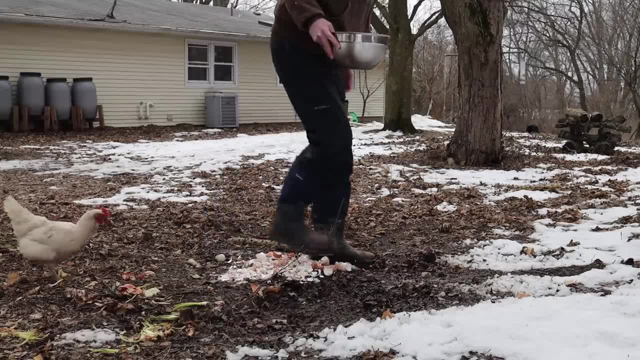 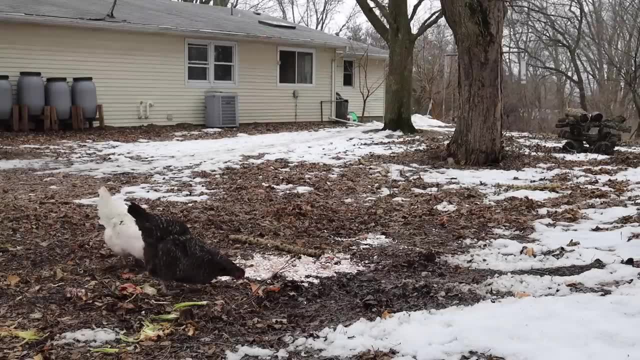 in that the chickens give us these eggs that nourish us, that we eat in our meals, and then we go ahead and give them back the eggshells to nourish them, to give them the calcium to keep the cycle going. It's just, it's a really cool thing. 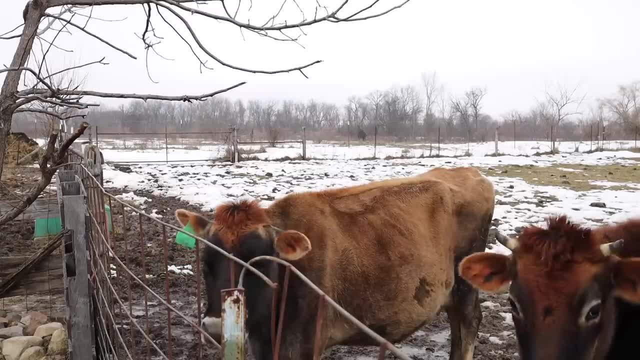 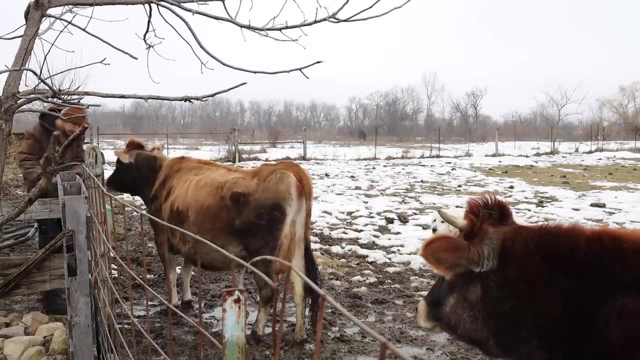 and we get excited about that. But you can feed your chickens eggshells. we just dump them out there, crush them up a little bit and they go to town and love eating them. And right now, since we are in winter and we are feeding hay to our cows, 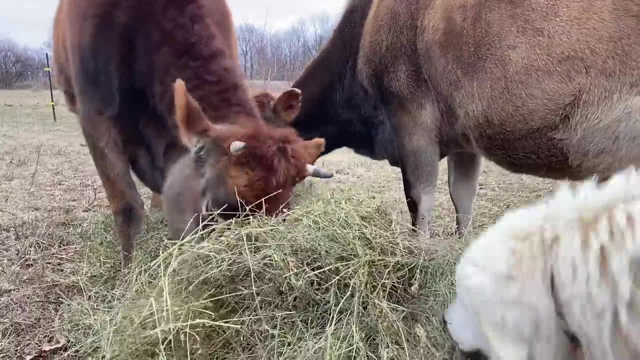 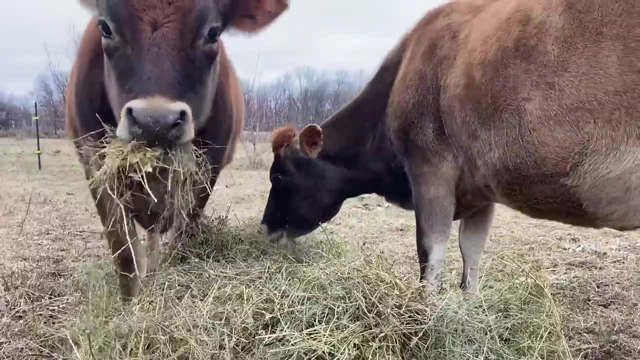 we have to give them hay three times a day. so while he's out there giving the eggshells to our chickens, he's also gonna give our cows their lunch portion of hay for the day. My cup overflows. That how it goes. 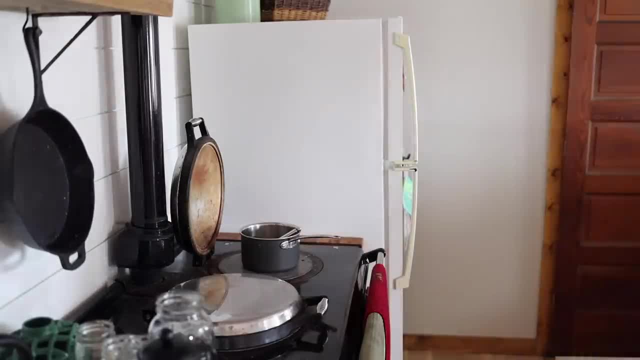 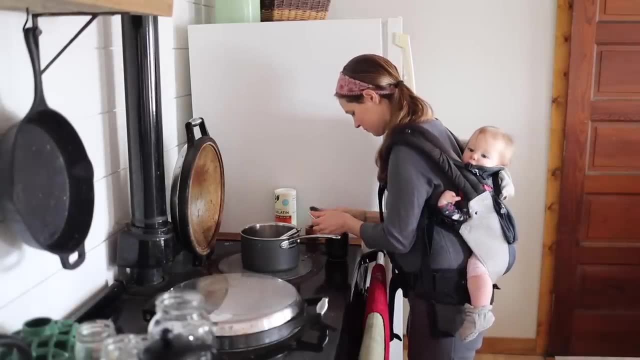 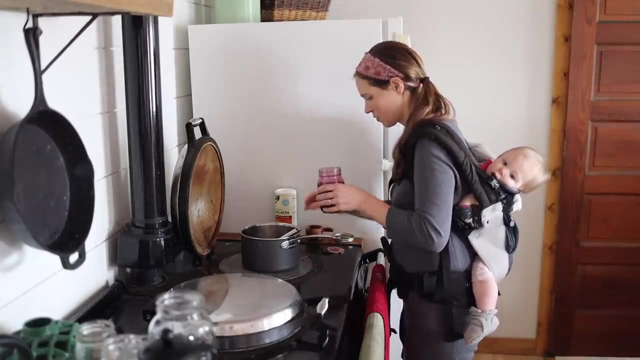 Now it does. The Lord is my shepherd. I shall not want to be in the house of daddy or the house of right hand. The other thing that we're gonna be making here today are homemade gummies, and we love homemade gummies. I think they sound like they would be complicated to make. 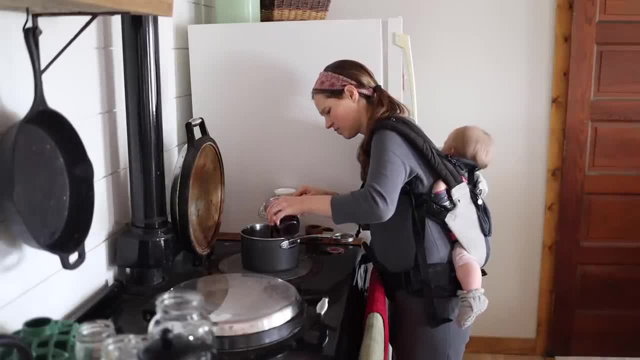 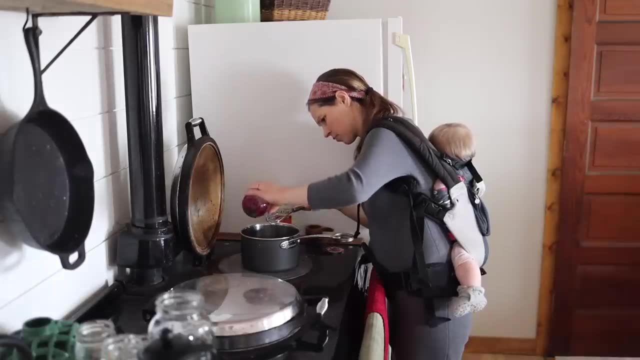 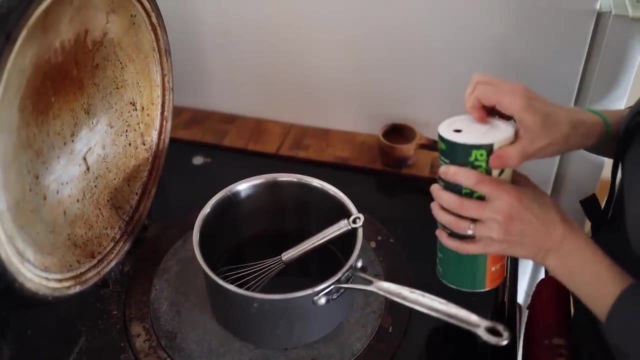 but they are so easy. They only use three ingredients and are really things that we always have on hand. We typically use either an elderberry syrup or a grape juice to make gummies, because those are things that we often forage for or we'll harvest from our farm. 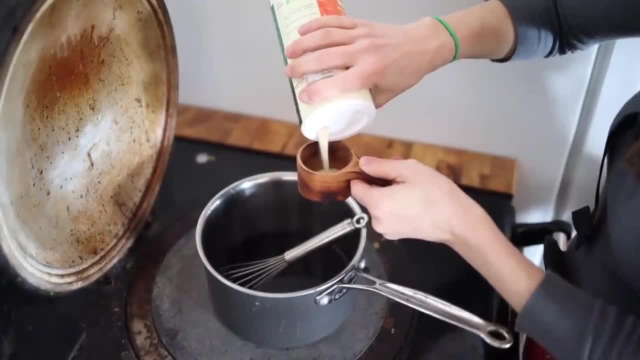 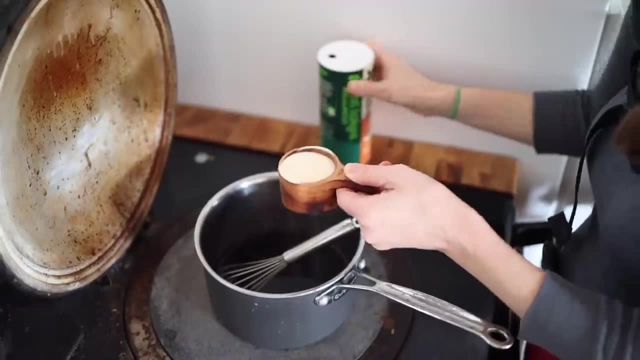 in the fall, and then I will can in these jars, and so we just always have these things on hand. Today, we're making grape gummies from our grapes that we have here on our property, that I turned into juice and that I canned this fall, and so all you're gonna do 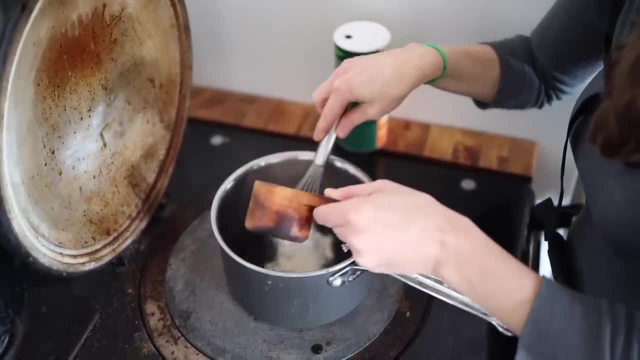 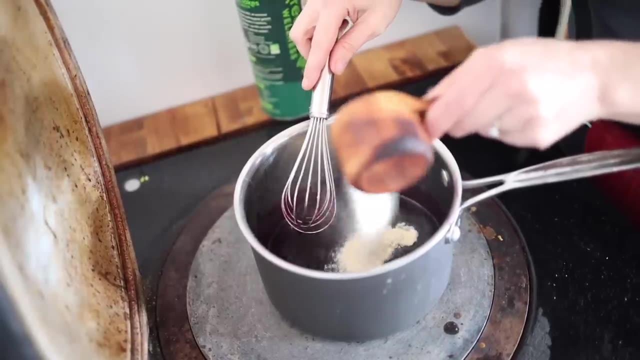 to make gummies is you heat up whatever that liquid, that juice is that you're gonna be using. You could also use something like lemon juice, or there's so many different combinations you can make of gummies- but you're gonna heat up that juice. 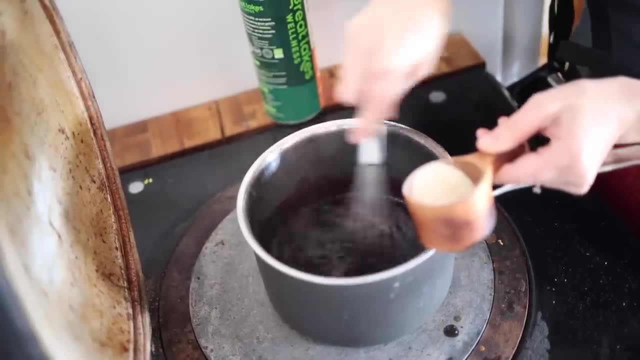 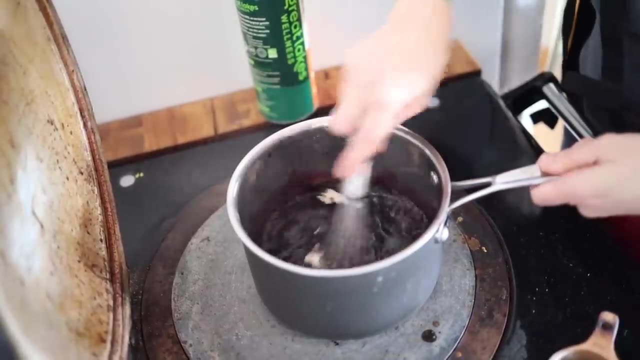 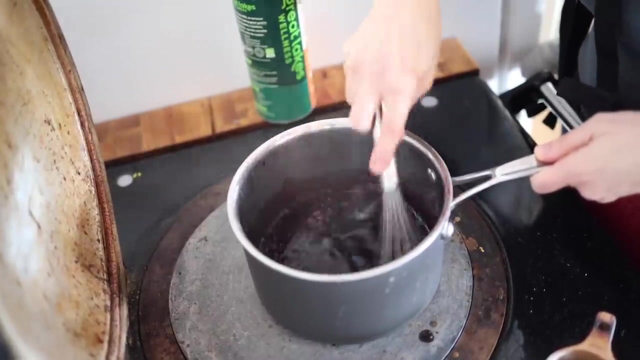 So we're gonna pour our grape juice into a little sauce pan. Once that's warm, we're gonna add in gelatin, and so I like to get the Great Lakes gelatin. I can link below the gelatin we use. but gelatin it's full of protein and it's really good. 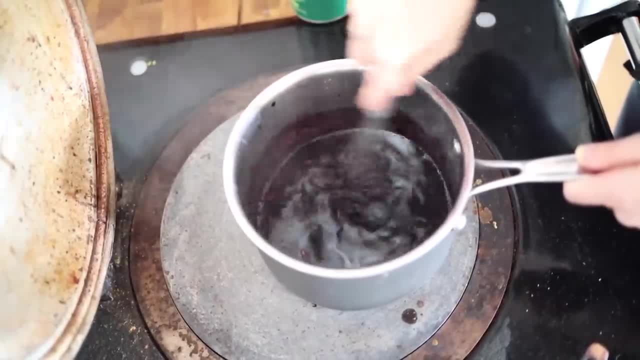 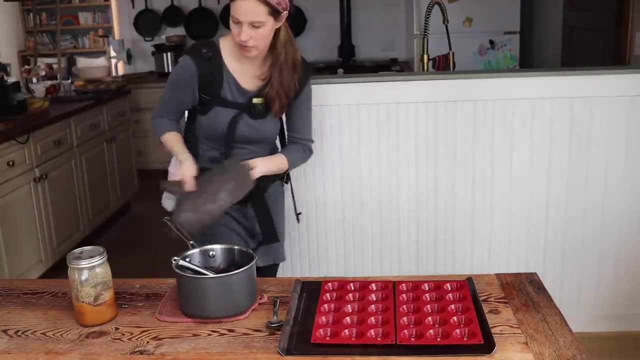 for your digestive health and it's just a really nourishing food, and so you add: it's just a really nourishing food and so you add, you add gelatin to it, mix it up. I like to do it with a whisk so that it doesn't get. 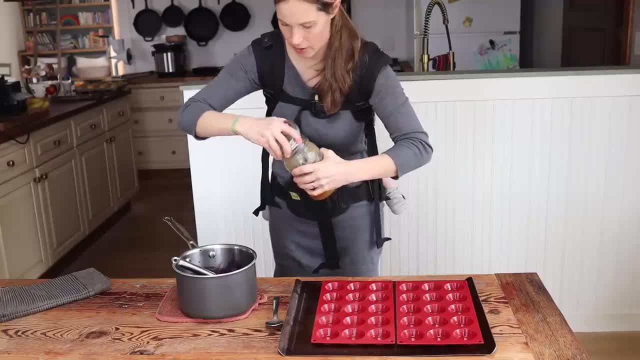 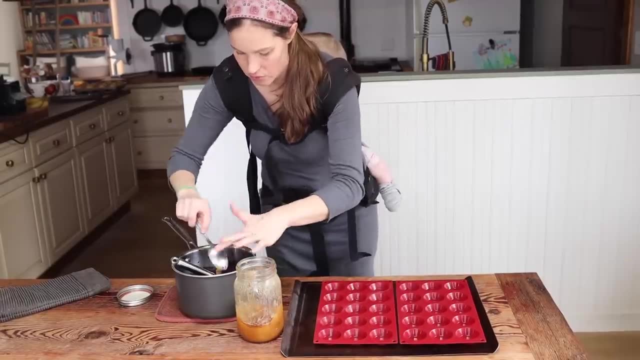 it can tend to form these little clumps. so then you get little gelatin clumps in your gummies. So if you use a whisk to really mix it around, good, you don't get those clumps, and so mix that together Once that's all warm and the gelatin is mixed in. 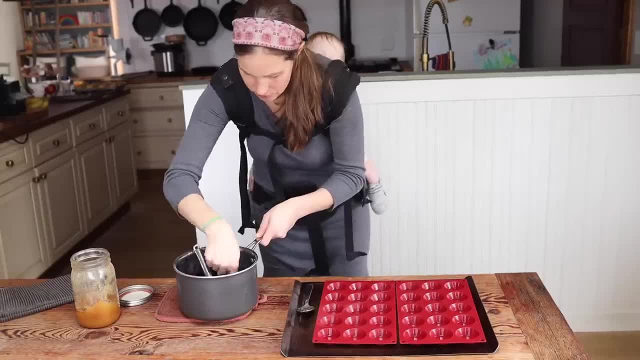 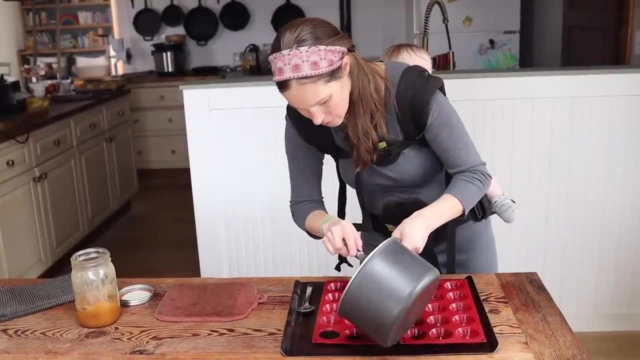 pull it off the heat and then I add a little bit of either maple syrup or honey to the pot until it's just the right taste. You just need a little bit Like a quarter cup to add to those gummies and then mix that all up and then you pour them into. 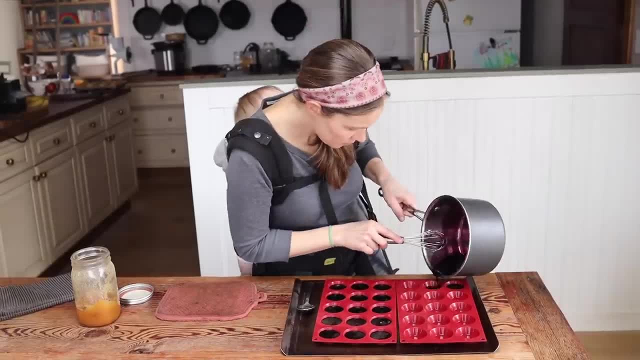 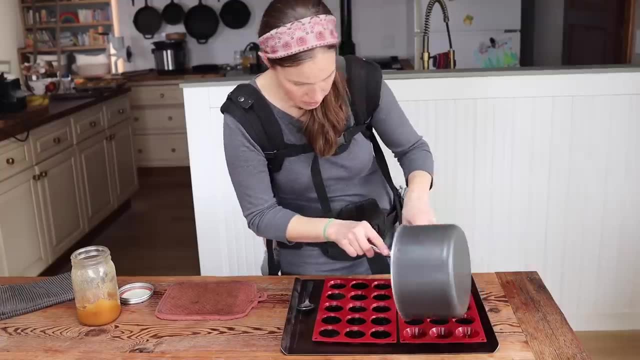 I like to use these little silicone molds that we have. You can get fancy. They have ones that look like little bears or little stars. if you really want to get fun with your gummies, and kids would totally love that. We just have these little small mini muffin silicone cups. 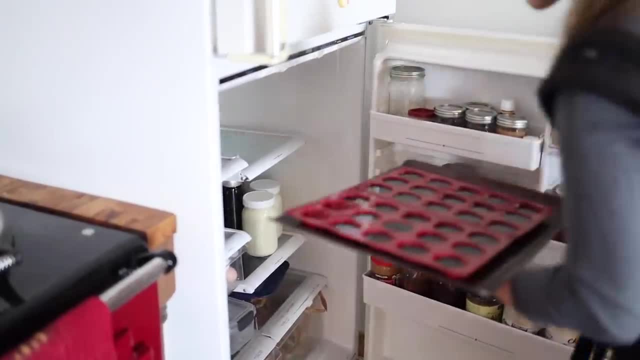 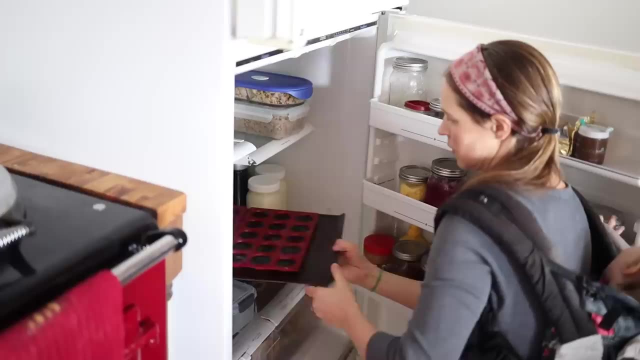 and so that works. I pour them into there and then, once they're filled up, you just put that in the refrigerator to. you just put that in the refrigerator to get firm like a gummy, and that's it, And they're ready to go. 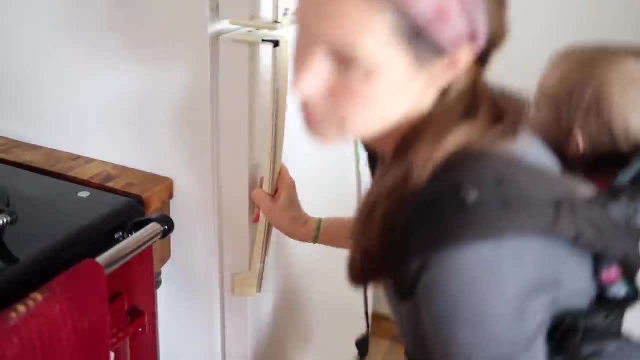 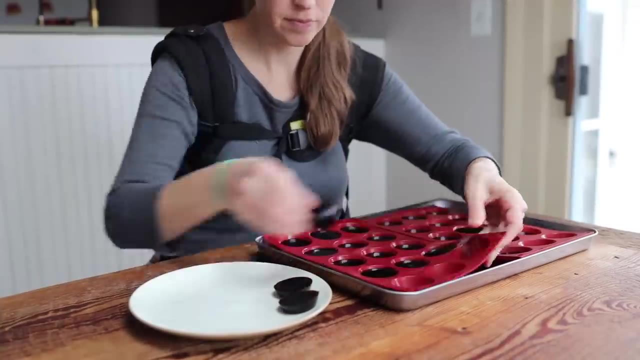 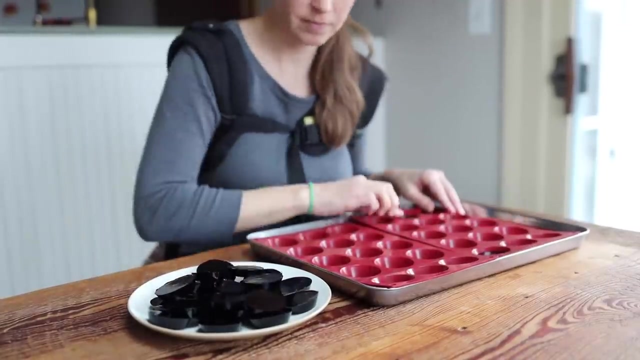 Gummies make a really easy, nourishing go-to snack, but for us they also double really well as a dessert. So if our kids are looking for like a little sweet treat to have after dinner one day- which we do sometimes- then really gummies are kind of our go-to for that. 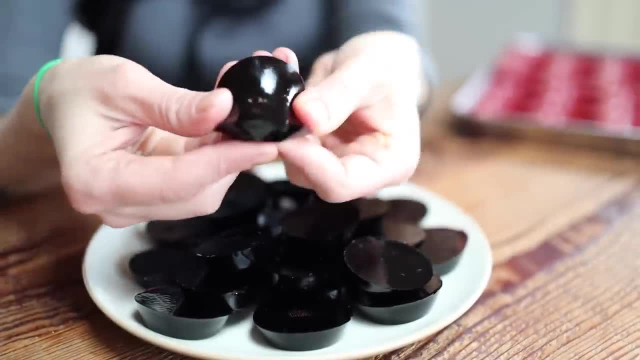 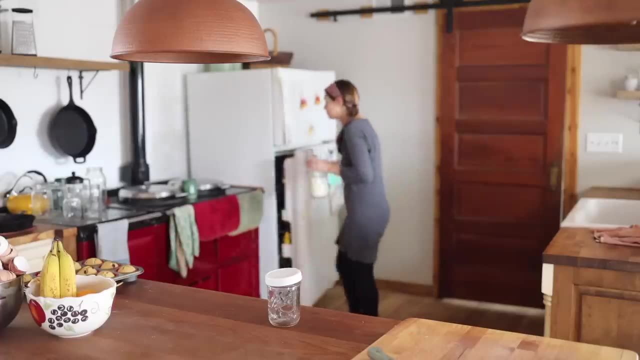 And I love that because they're just a really nourishing but also sweet and satisfying dessert option. All right, so the last snack option that we always have on hand is dairy. So we have a family milk cow on our property and dairy is big for us. 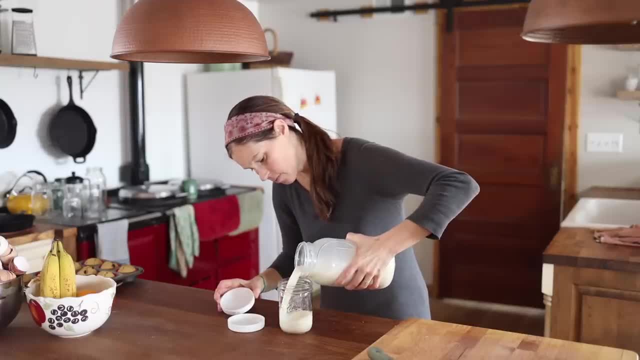 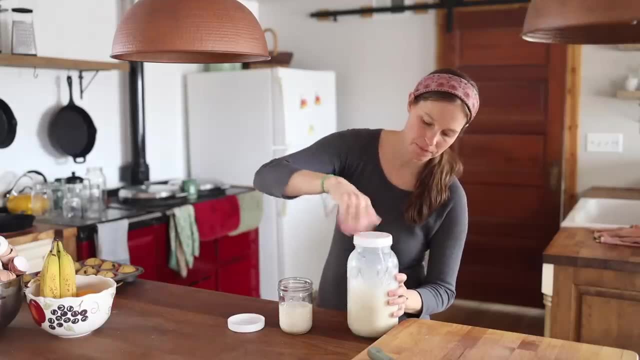 And I love dairy any time of the day, but even as a snack, because it's such a balanced food that it has a good amount of protein, carbohydrates and fat, And so it's just really nourishing, It's really satisfying as a snack. 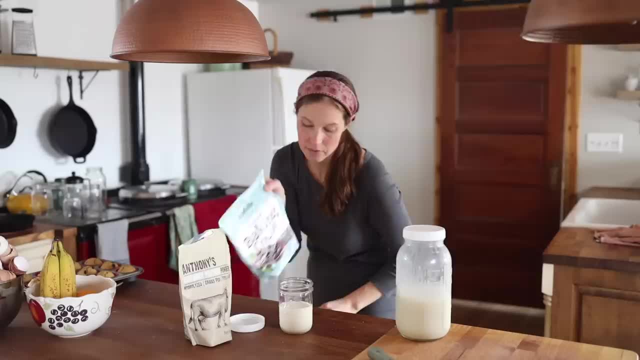 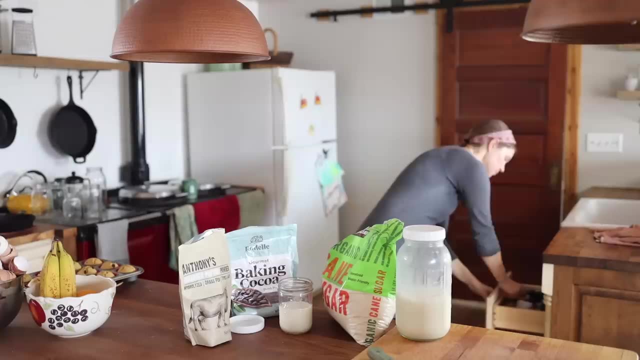 Like I said before, if our kids get hungry between meals, the thing that I always say that they can have is a hard boiled egg. The other thing that I always say that they can have is a glass of milk. So those are kind of our two main. 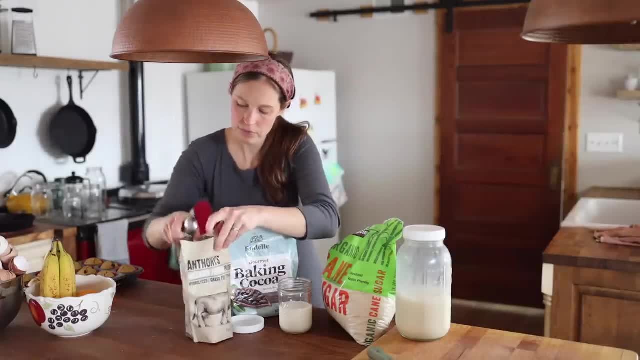 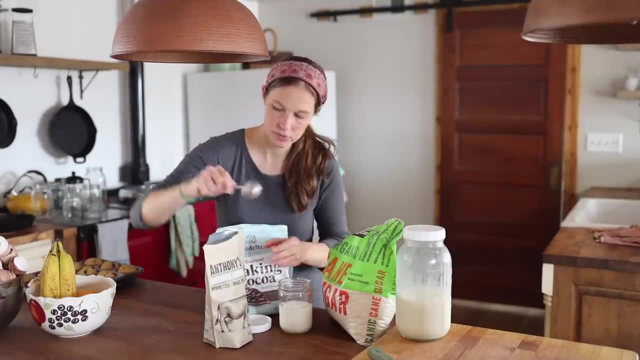 you're hungry, great, There's hard boiled eggs and there's milk and you can have either one of those. So dairy is just a big one for us. but there's also so many ways that you can do dairy as a snack. You can do yogurt. 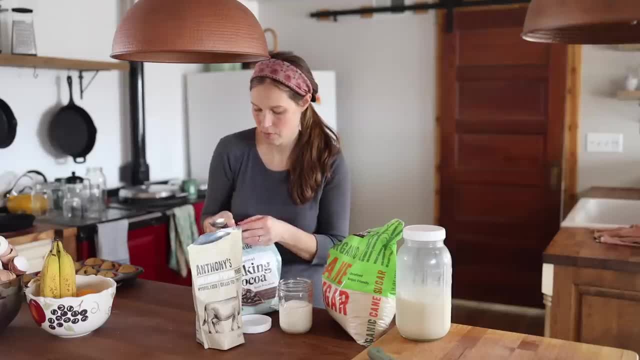 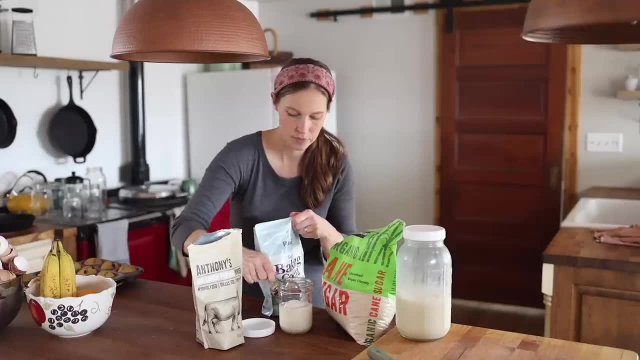 You can have a little piece of cheese, You can do a straight up glass of milk or, in the last year or so, a way to have milk as a snack is actually to make this chocolate milk When I was pregnant with our daughter last year. 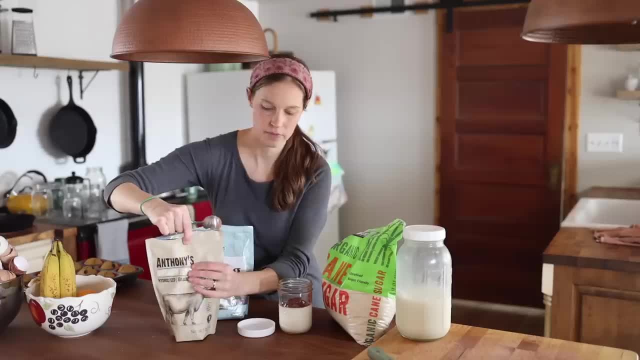 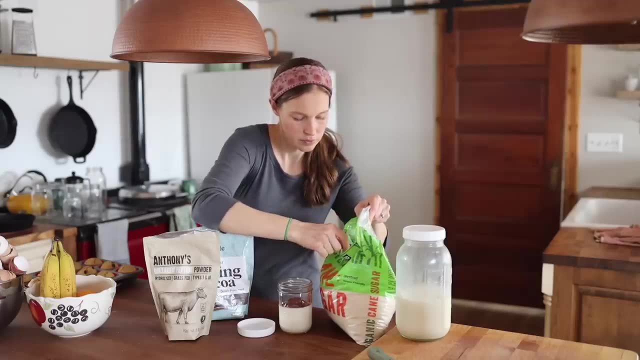 I craved chocolate a lot, And so I started making this chocolate milk as my like go-to after the kids went down for their naps and I just wanted a few minutes of peace and quiet, And then I would make this glass of chocolate milk. 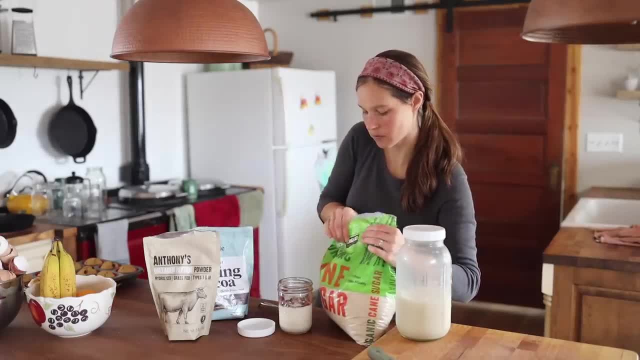 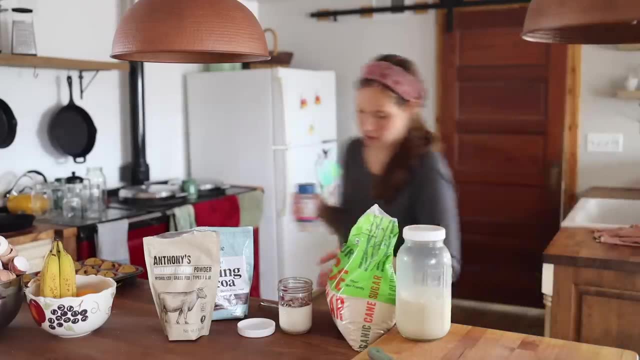 to enjoy during that time And that just became my routine and my thing. And while I did it almost every day when I was pregnant, I don't do it every day now, but I will do it every now and again And I still really, really enjoy. 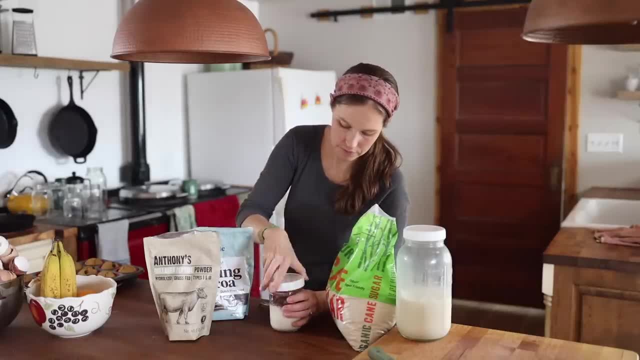 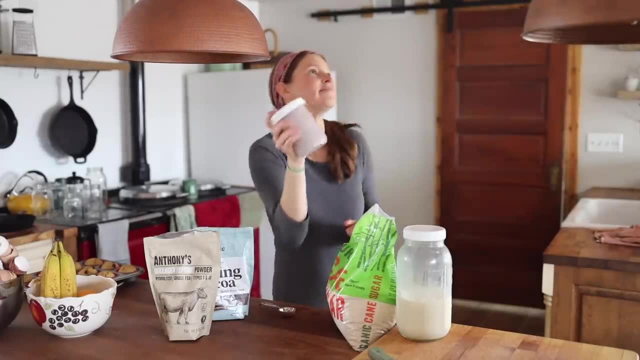 That is a little kind of personal, just treat and snack, but good, kind of just pick me up, unwind time if it's been one of those days and that is needed, And so to make the chocolate milk which I also have a recipe for below. 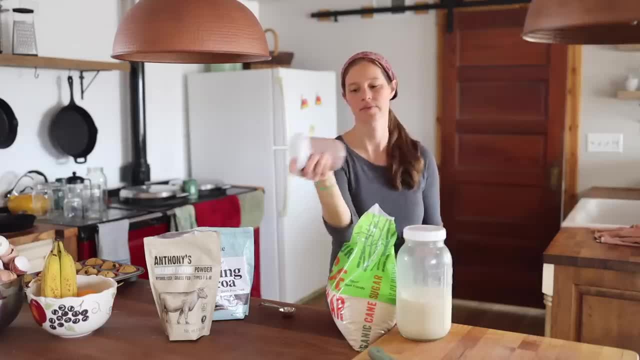 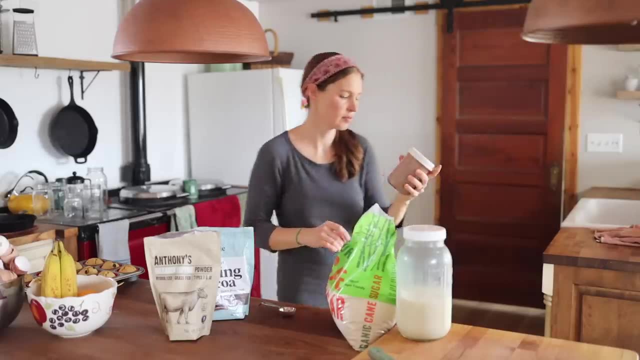 but it's really simple. I just use milk and then add a little bit of cocoa powder, a little bit of sweetener. You could do cane sugar, You could do honey or maple syrup, And then I like to add collagen powder for the extra protein there. 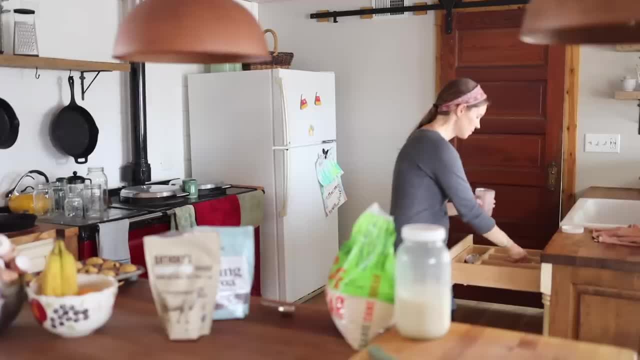 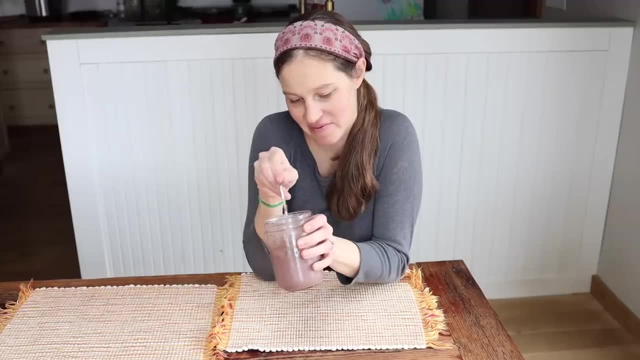 I'm always trying to get more protein in my diet. And then you just shake that up like the Dickens. I just put them in a Mason jar with a lid and just shake it like crazy And that's it. It's a really good, yummy and nourishing snack. 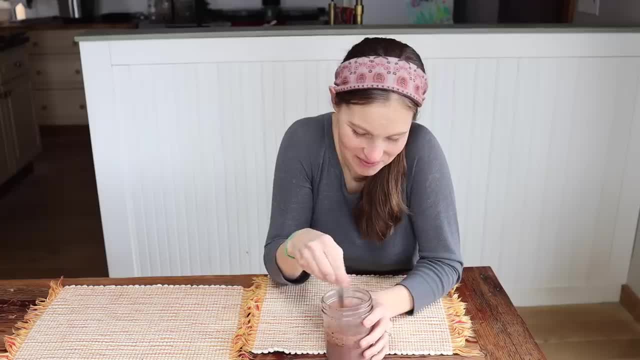 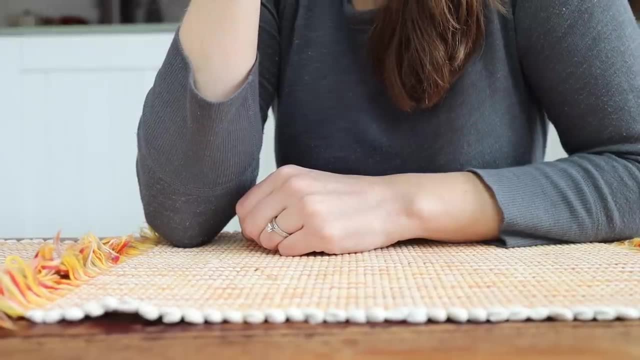 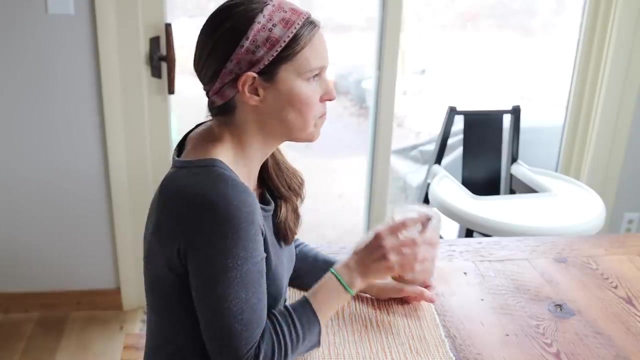 Well, we will always place the biggest emphasis on making nourishing, solid meals for breakfast, lunch and dinner Every day. having some of these ready to go, kind of more snack foods- on hand all the time can just be really, really helpful to making smooth days.